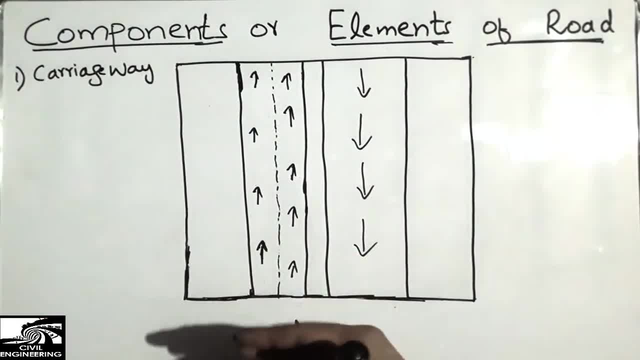 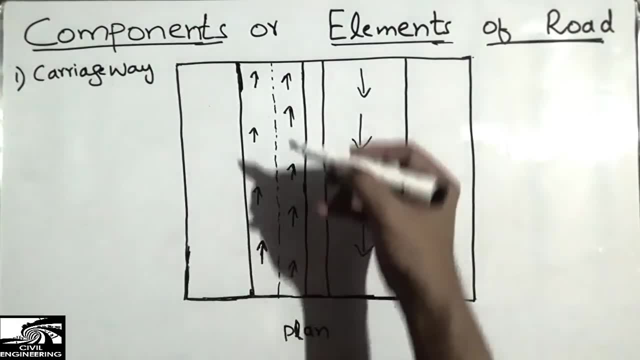 carriageway. Carriageway is the way in which the traffic moves freely in one direction, or maybe in both directions. For example, this is a carriageway, but this is a two lane carriageway, because one lane is here and 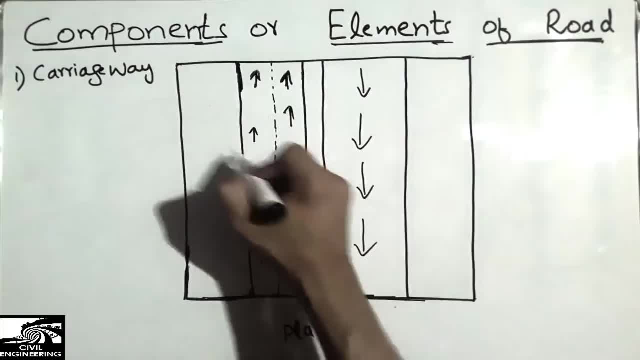 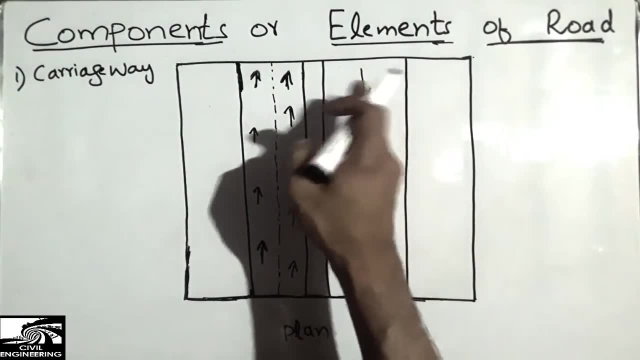 one lane is here. This is a two lane double lane carriageway. This is the single lane carriageway. The traffic is just moving in one lane. There is no other lane, So we call it the single lane carriageway. This is a double lane carriageway. 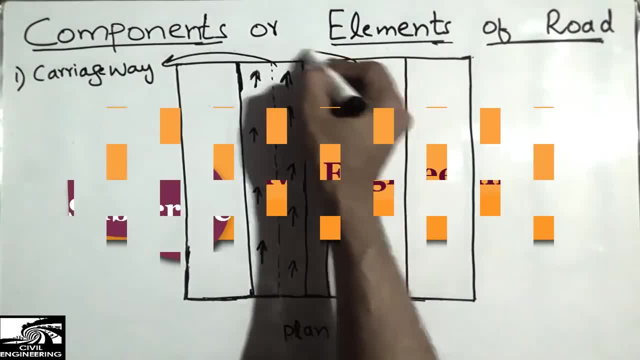 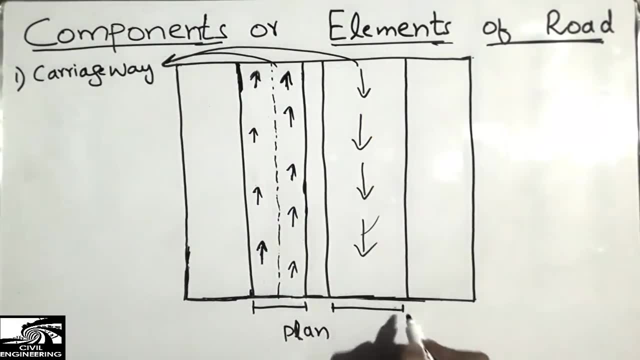 single lane carriageway. So these are the two carriageways Right And the length generally of these two carriageways is: the single is 3.8 meter we take and the double carriageway is 7 meter generally. 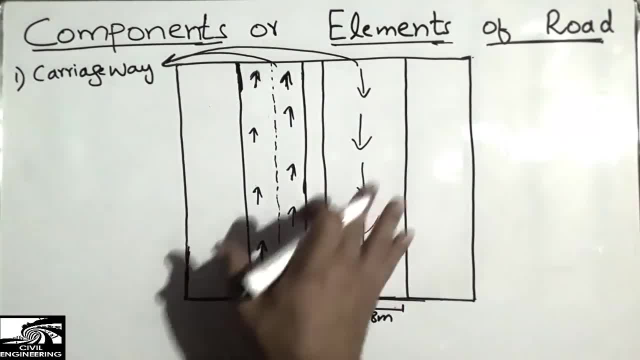 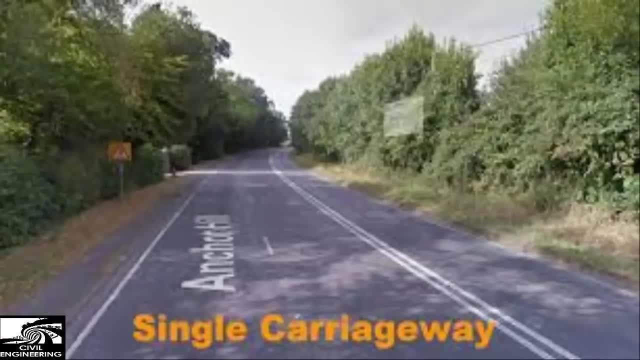 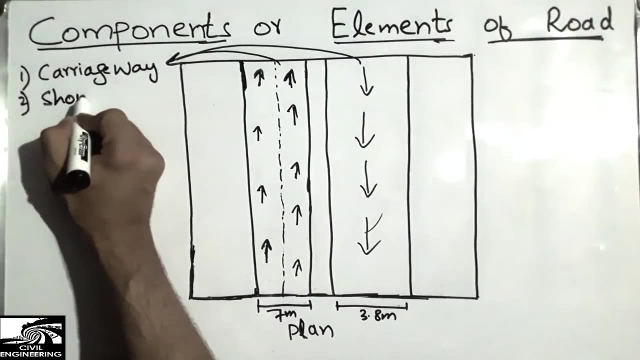 according to the standards, Right. So the first one is the carriageway in which the traffic can move easily without the disturbance of anything. The number second one is the shoulder. Sometimes it's also called hard shoulder Right, So the shoulder is. 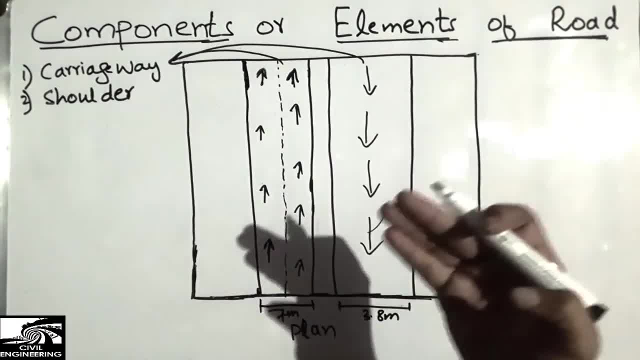 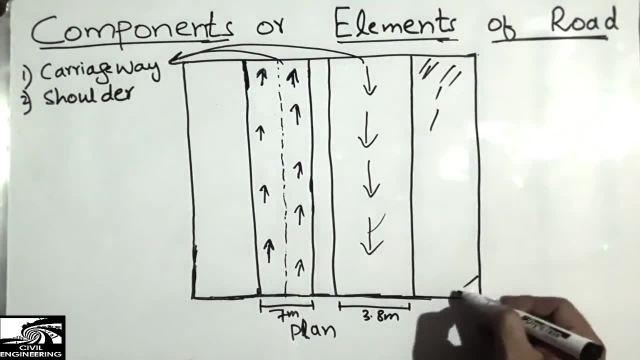 the part is the emergency part of which the vehicle can stop at any time at the sides of the carriageway. So these are the shoulders provided Right. These are the shoulders On the right side. these are the shoulders. This is the shoulder On the. 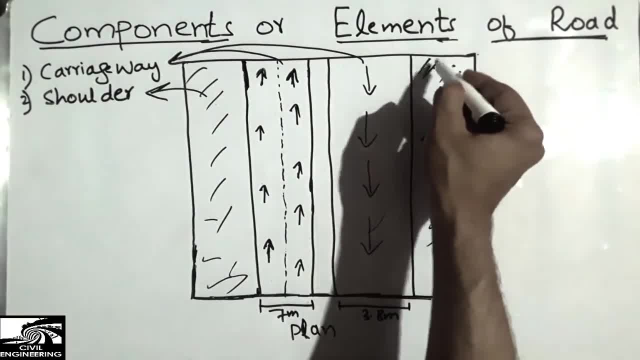 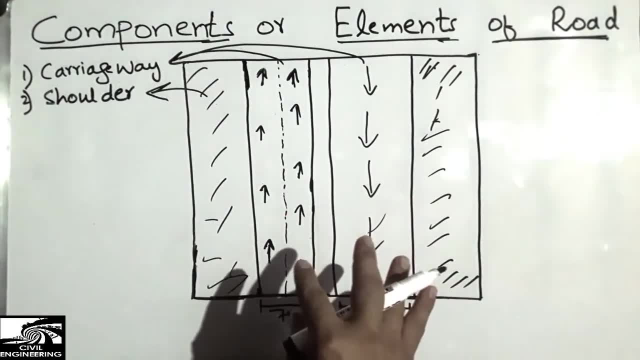 left side, right. It's one shoulder and this is another shoulder Right On the right side, And it's provided just for the emergency cases. some vehicle is going to stop, so they can stop and it can move here, and this can move here and can stop there for emergency. 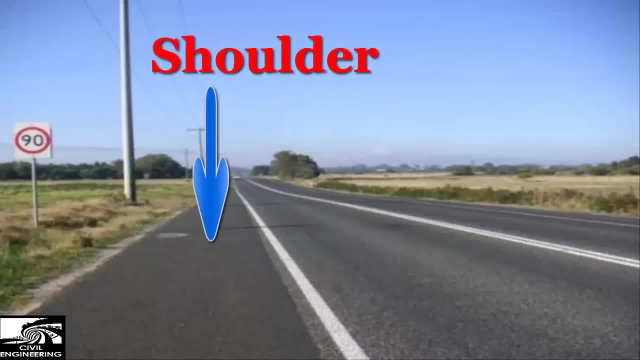 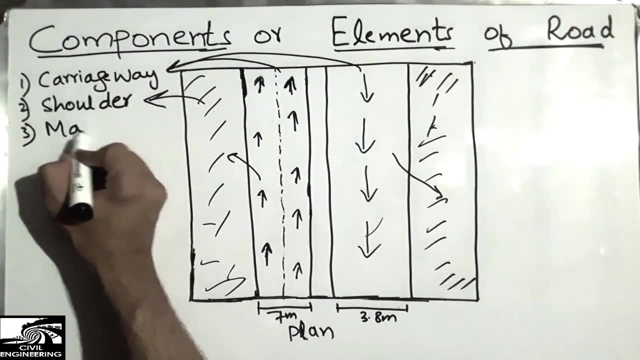 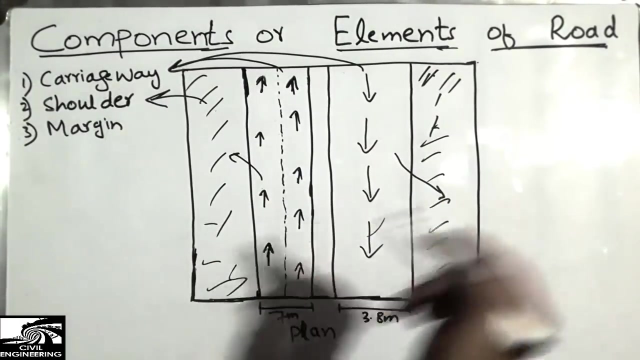 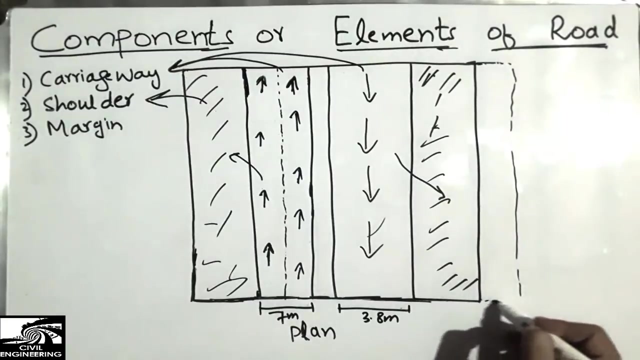 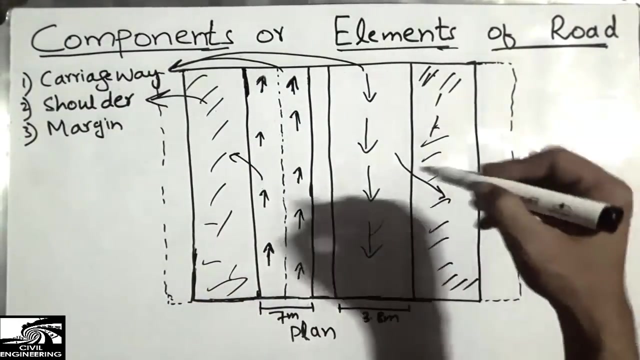 purposes Right. So number third one is the margin. Margin is the type of the component of the road which is provided after the, the, after the shoulder right, a small portion of the road is provided here. we call it the margin. it is the last part of the or its last part of the road. we 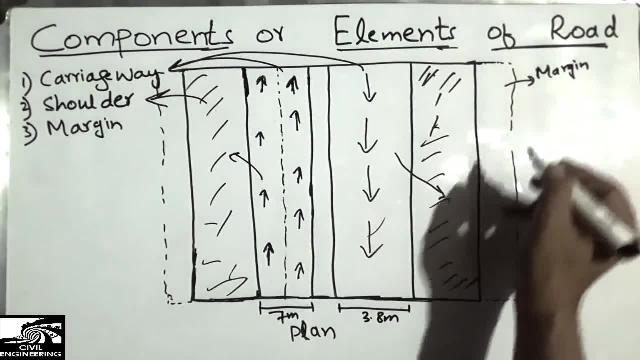 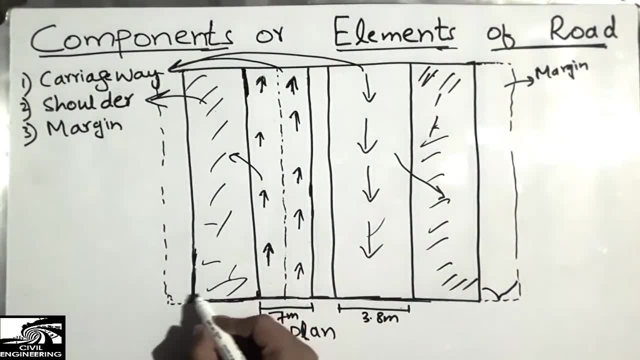 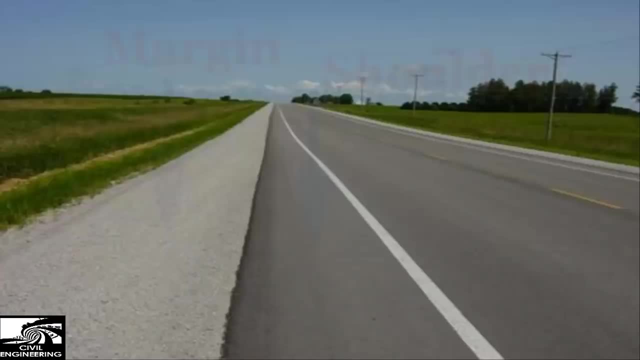 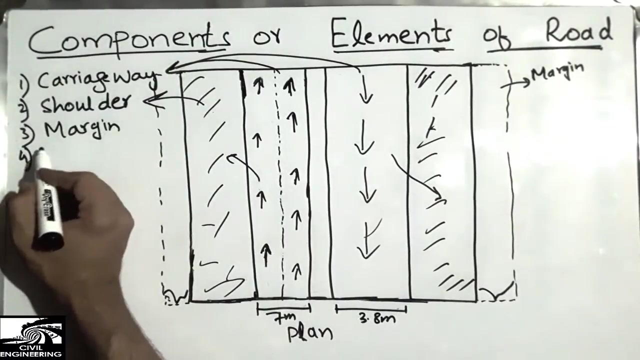 call it the margin, and this usually provide for the drains of the water. the water usually sometimes moves here, drain like water passes into this portion. it is the last part of the road. let we call it the margin. number four is the number four. there is a combination of these two we can call. 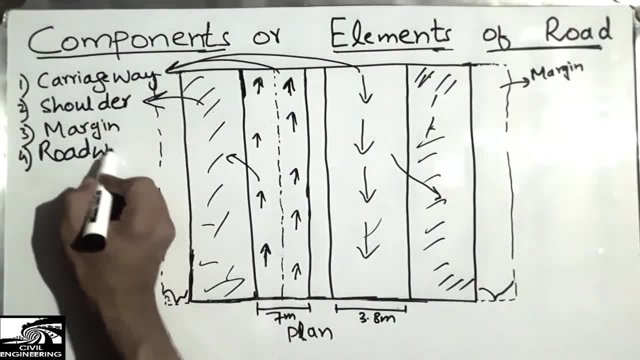 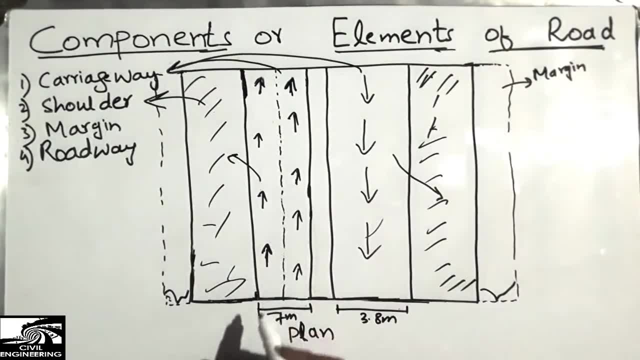 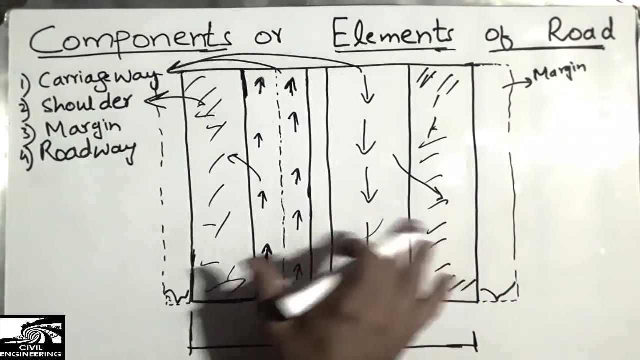 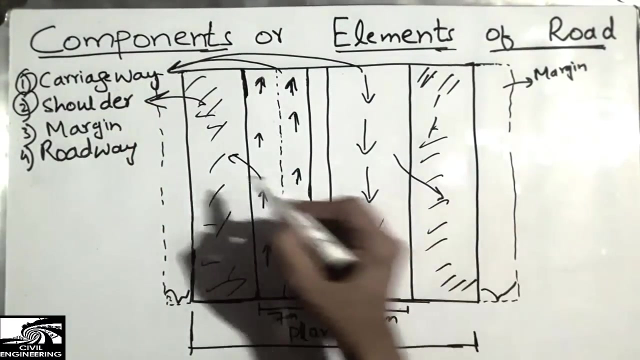 it roadway, roadway, roadway is the is the road consists of the from the shoulder- this is the shoulder, shoulder right- from the shoulder to the another shoulder right. it consists of shoulder and carriageway, the shoulder and carriageway. these both two we call is the roadway. so or we is the combination of what is the. 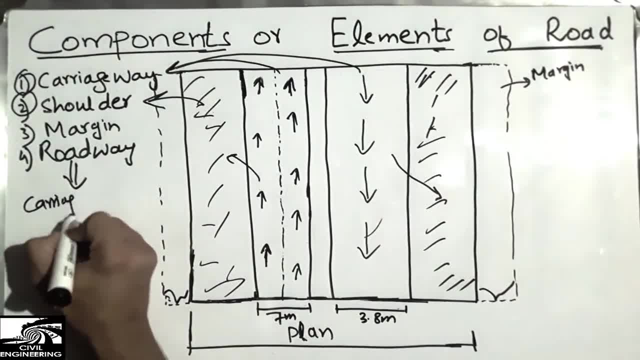 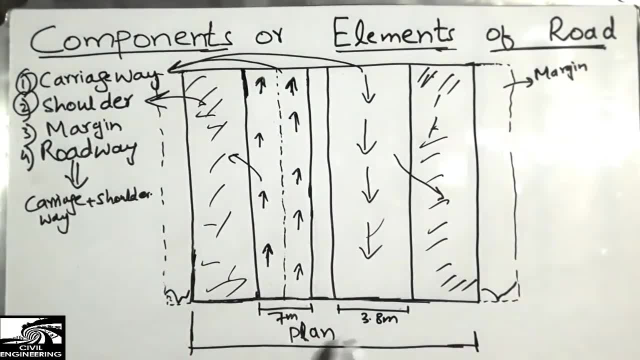 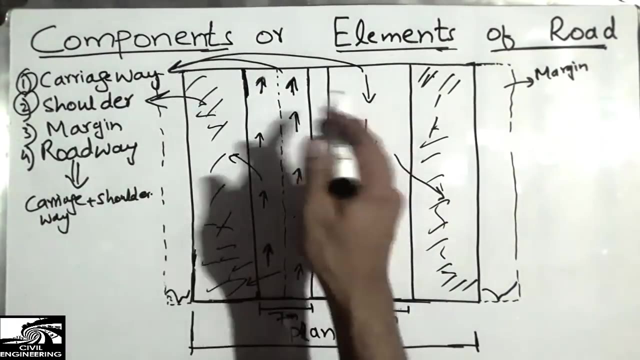 combination of carriageway and carriageway plus the shoulder. we call it a roadway, a right. so it composed both the uh, the carriageway, as well as the shoulder. so we call this uh road path. we call the this distance, uh, we call the roadway of the road number. fifth one is the right. 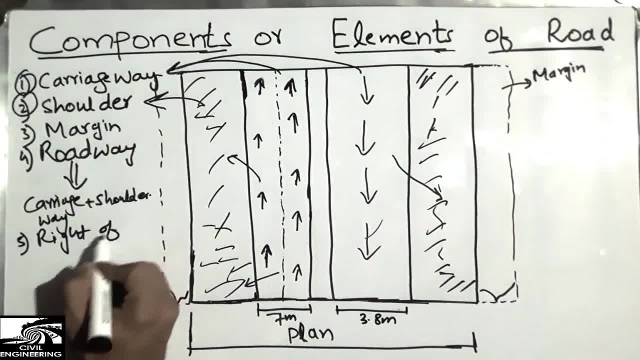 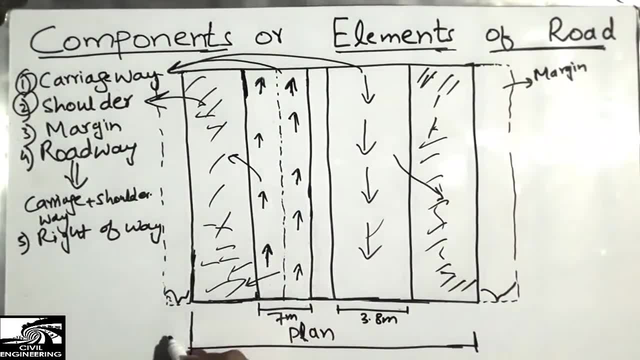 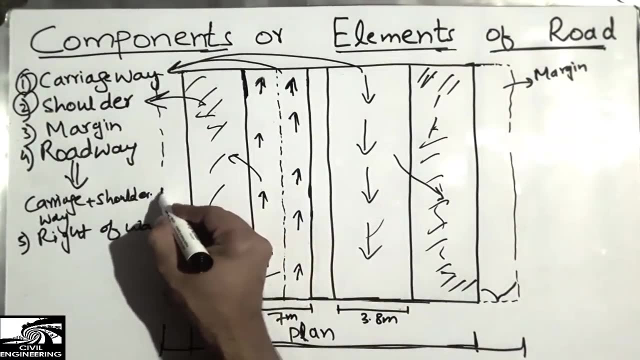 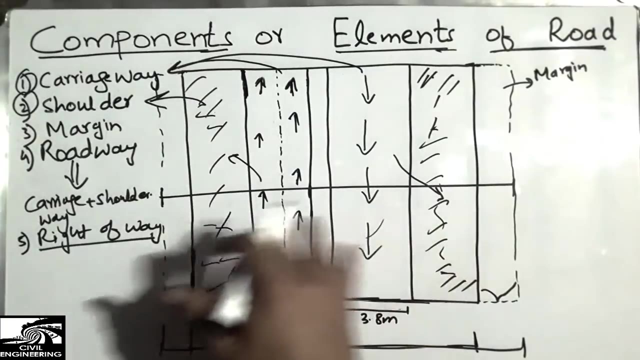 of faith. right of faith. right of faith is the uh is the whole length of the road from the margin, from the margin to the another margin, the whole length of the road from this margin to this margin we call the right of faith. it's the longest length in the road across this direction. 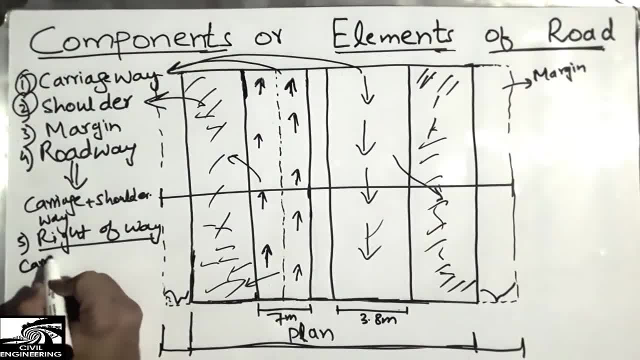 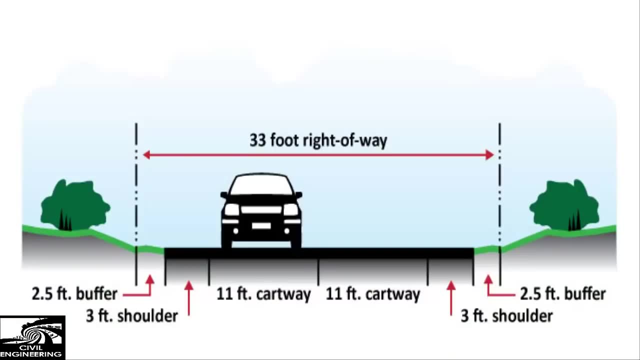 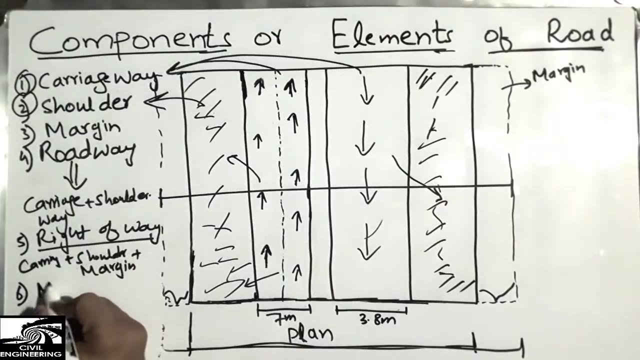 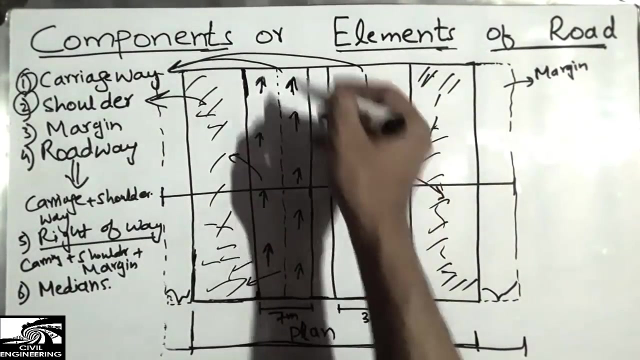 we call his right of faith. it's a combination of territory plus shoulder, plus margin. it's the combination of all the parts, of all the in the root components, to be called the right of way. so number six is medium medians. the median is provided between the opposing road traffic way, for example. 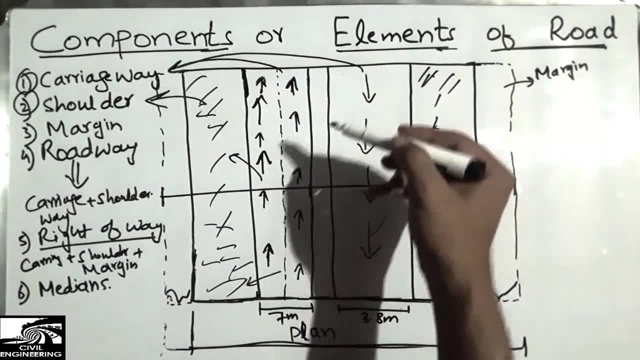 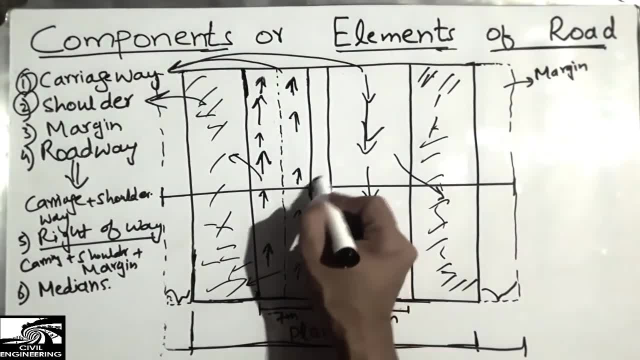 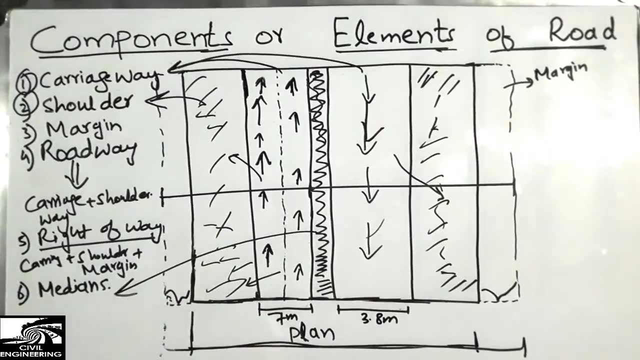 this lane car moves in this direction while these cars move in the opposite direction, so they are separated by a type of way, a type of separation- so we call this separation path- is the median right. this separation path is called the median, provided it even motorway or the highway. 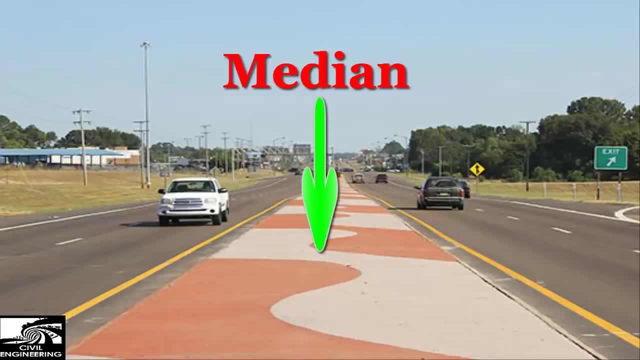 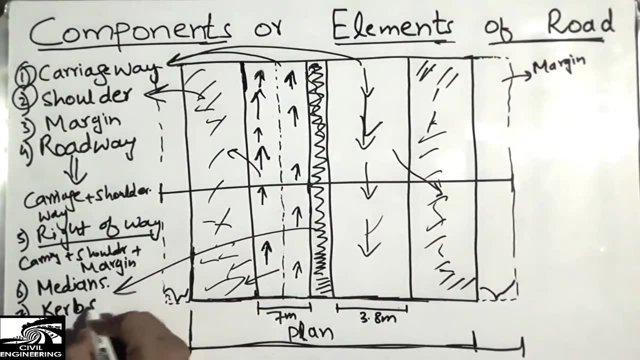 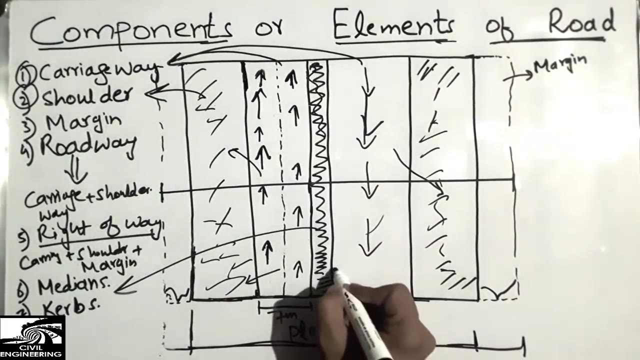 number 7 is the curves. the curves are provided along the median. along the median. you can also see in the pictures i provided, each picture of these tums, these components of the road. they are provided to the road out the medians right and both the directions called. 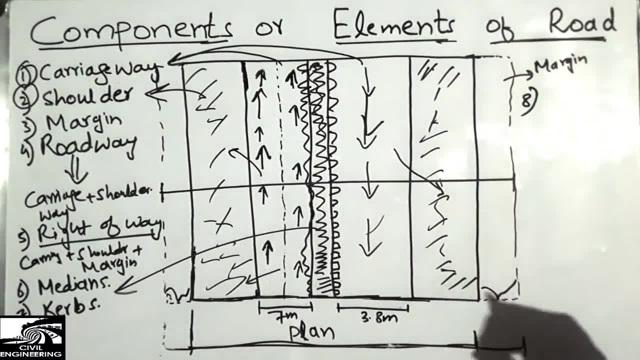 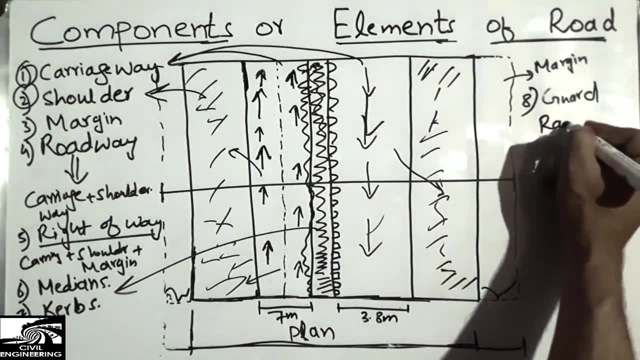 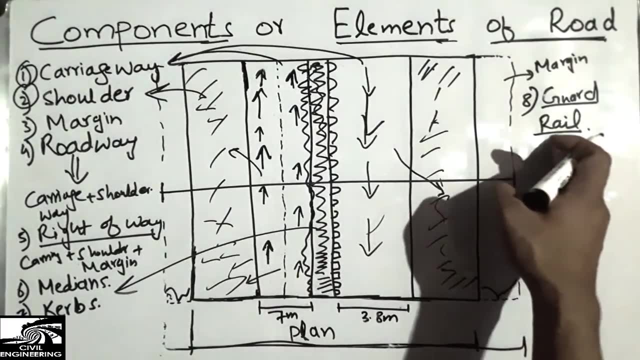 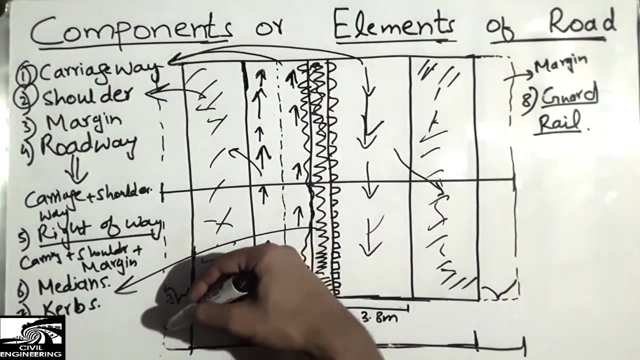 and the number last one I can set. last one is the not last one guard rail, but the second last one guard rail. these are also be important, provided mainly, and the heavy hilly areas. they are provided to support the car or the vehicles from accident, from accidents, and some more. some parts are provided here you will. 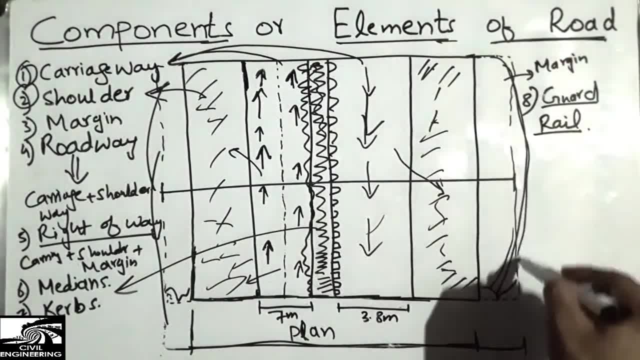 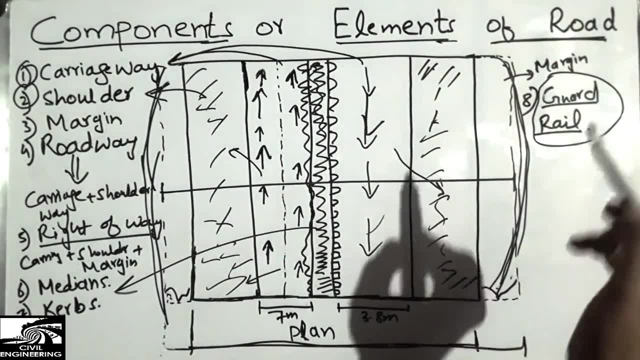 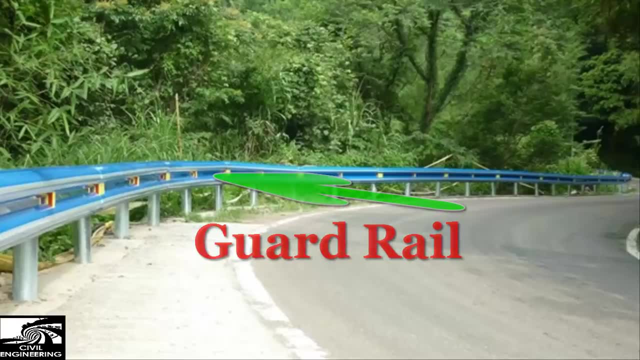 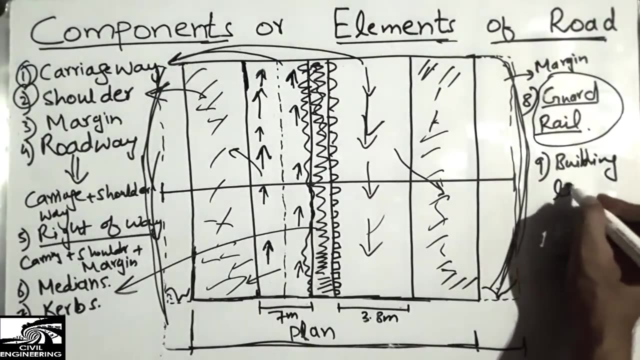 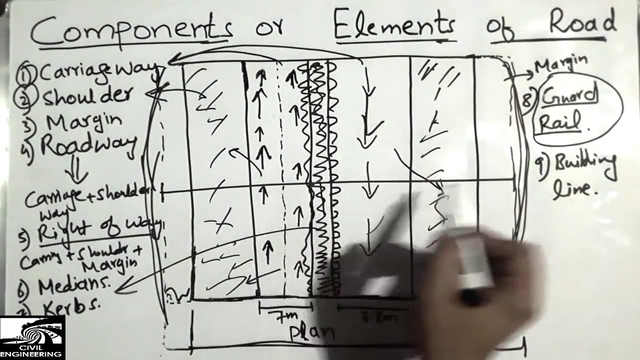 see images that some or some rails are provided at the last portion of the road vehicle is the guard rail. they are provided to support the vehicle, to guard the road vehicle right. the last one is the building line building line. building line is the distance from the center of the road. the center of the road, sorry, the center of. 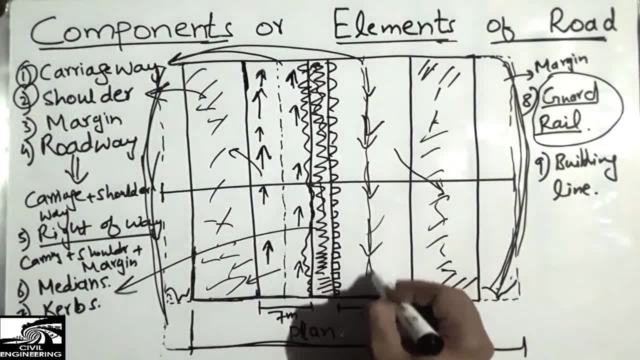 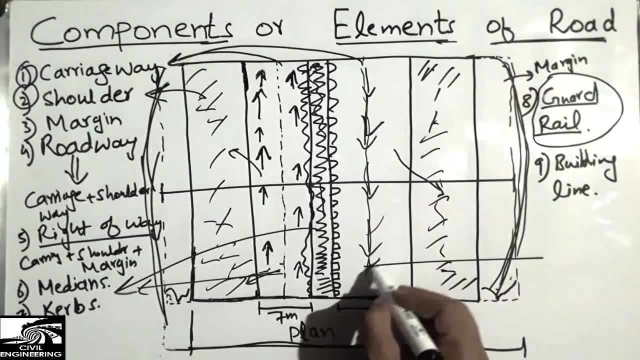 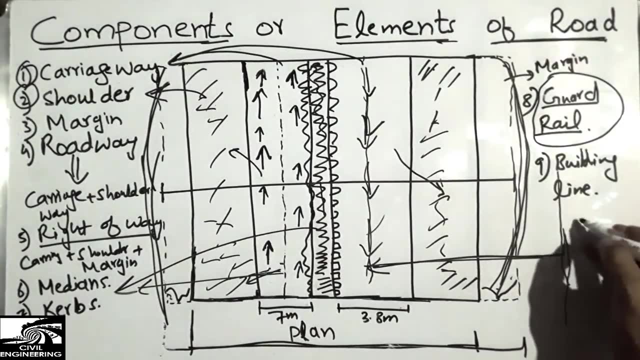 the carriageway, the center of the carriageway, and this is the another center of the carriageway right. so the distance from the center of the carriage way to the to the building site, for the example, there are buildings constructed here. they are buildings right. homes are. 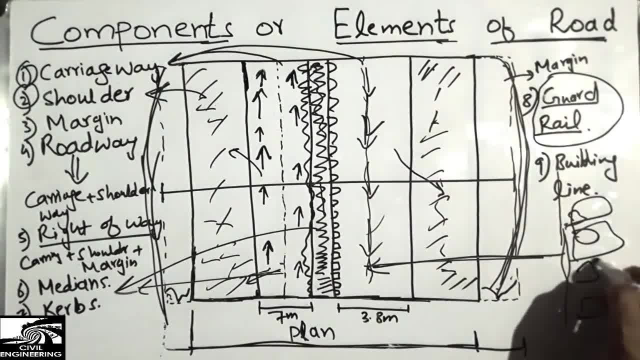 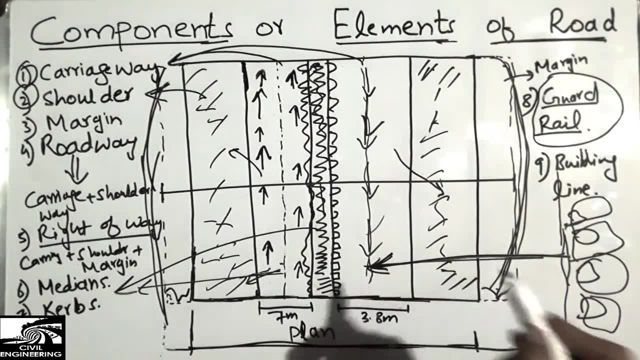 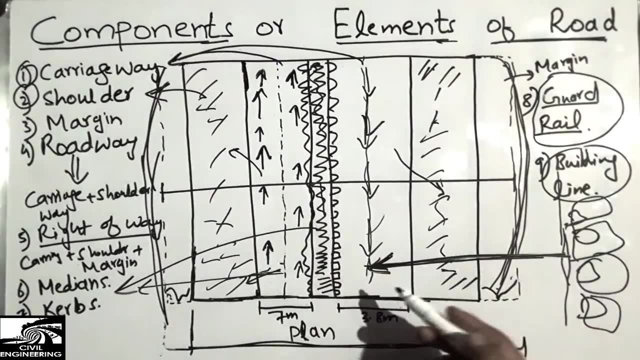 maybe another buildings, maybe some petrol pumps or some other places, to the distance from the center of the carriageway to the buildings we denote and we call. this is a building line and it a different, according to different standards. Japan may provide it some, you know, at.